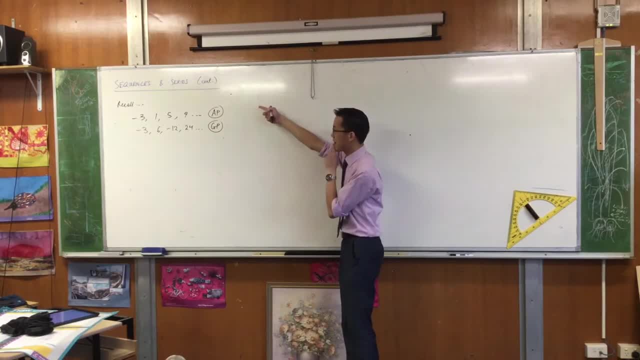 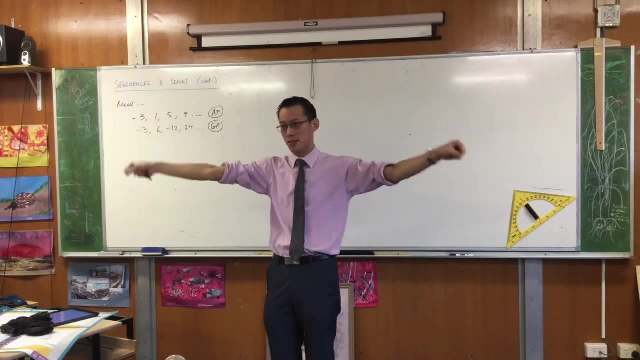 If you're like: oh, what's the sum, What's the series, If I take the first 1,000 of these, or a million of these, you for an AP, do you remember? You pair up the terms. Oh, I'm sorry, You pair up the first and last, the second and the second last, and so on. 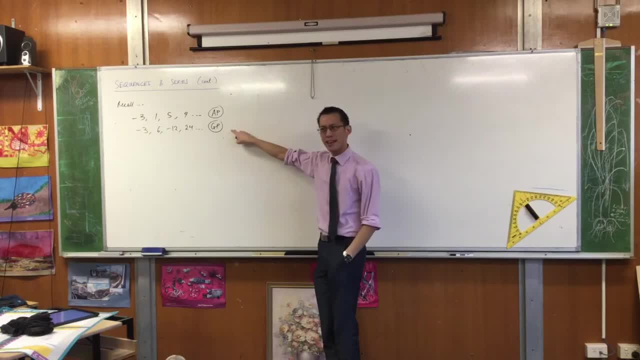 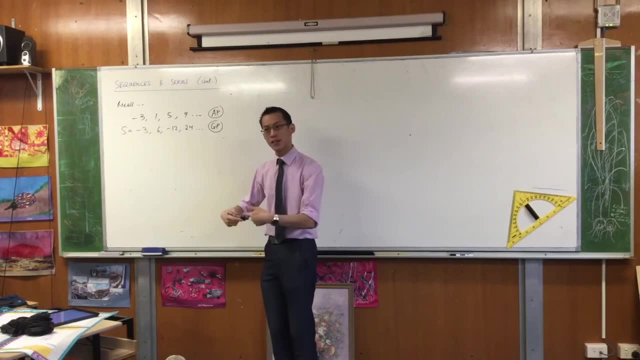 Everything's nice With this one. do you remember what we had to do If I said: okay, here's a series, a sequence, right? If you multiply everything by that common ratio, right? So if I say, what did we say? the common ratio was: 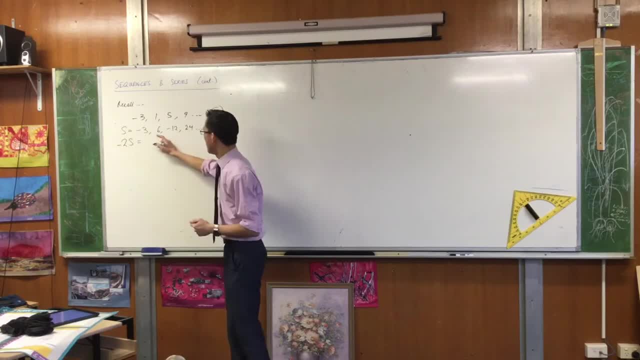 Negative two. So if I multiply everything by that, then every term turns into the next term, right? So this negative three will turn into a six, This will turn into a negative 12. This will turn into 24, and so on. okay, 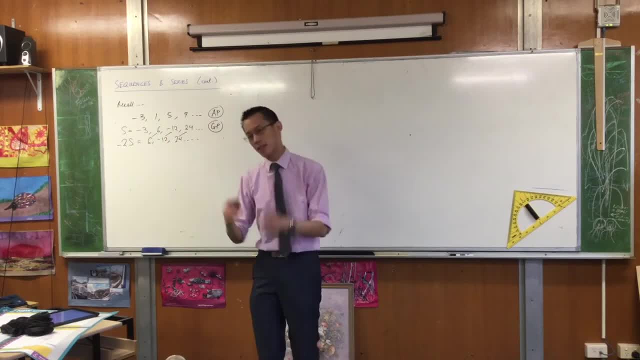 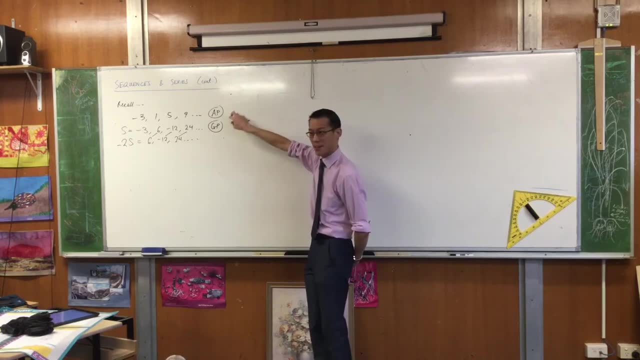 And because you can match up these terms, you can again find the sum of the series in quite a nice neat way. But not all sequences in the series are APs or GPs. In fact, one of the important examples I gave you was this guy. 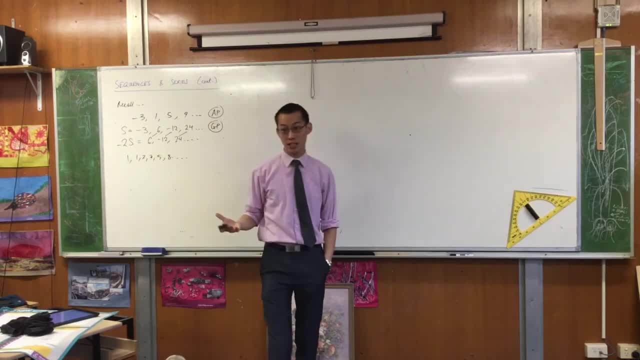 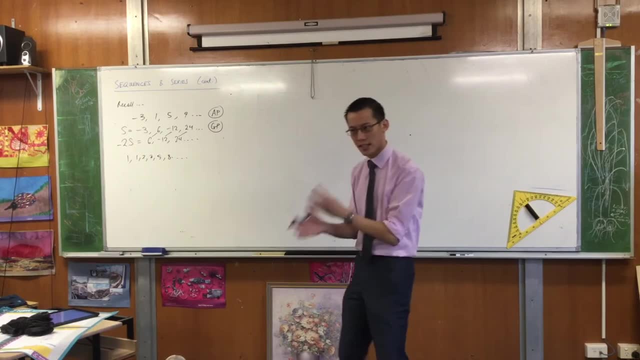 What's this guy again? This is the Fibonacci sequence, which is neither an AP nor a GP, but it's one of the first sequences you learn. It's quite easy to wrap your head around And it's quite simple to come up with different sequences that are none of these. 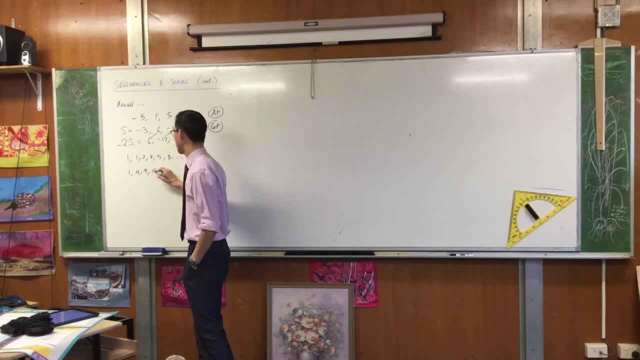 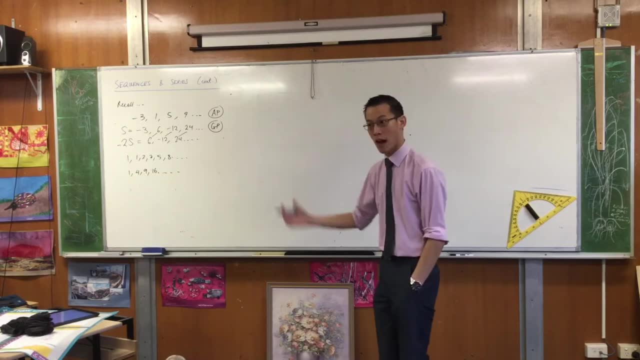 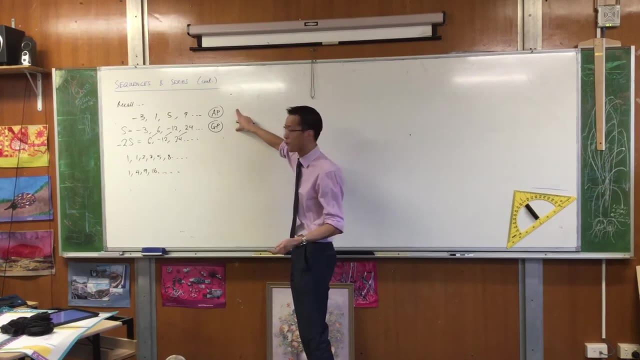 Here is another one, And I think this actually appears as again one of the questions in that chapter. This is the sequence of square numbers, right? And there isn't a common difference, There isn't a common ratio. So how do you deal with these things when you don't have the nice neat patterns that we established before? okay, 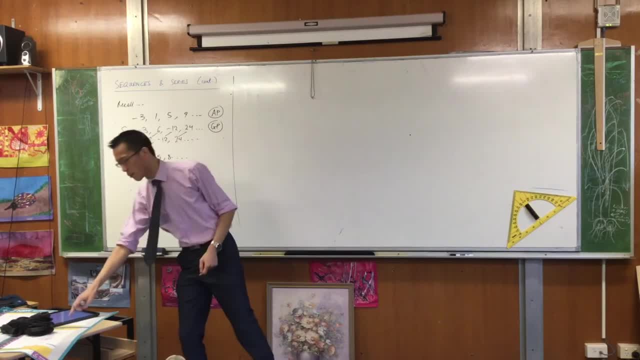 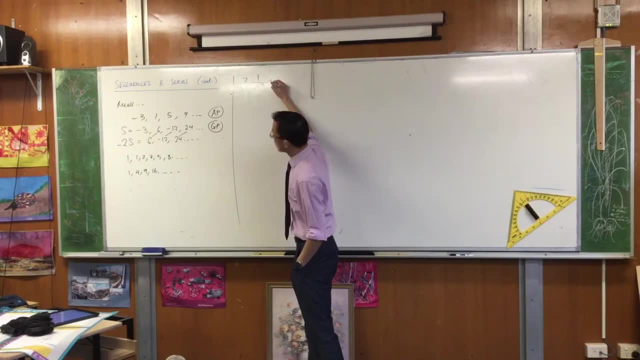 We're going to look for different patterns, So the question I asked you to look at- and it might help if we actually write this down first- was this one. It was number seven and it looked like this: What is it? 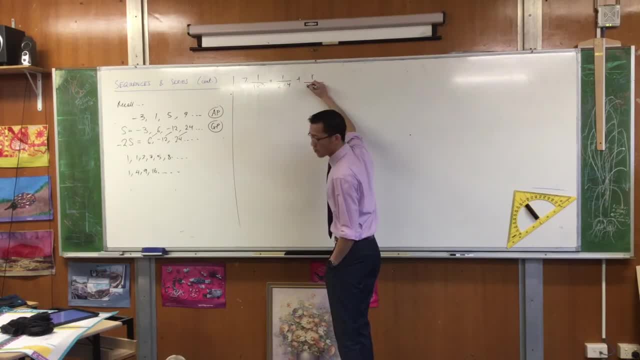 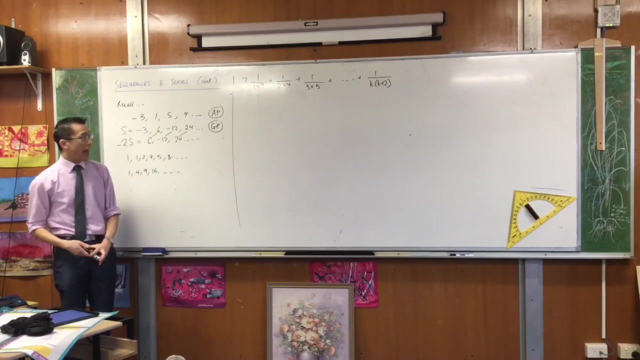 Three times five, I think. Yep, Okay, so this is what they want us to add up, and it just looks weird. It's all kinds of weird, right? There's no common difference, There's no common ratio, So how are we going to deal with this thing? 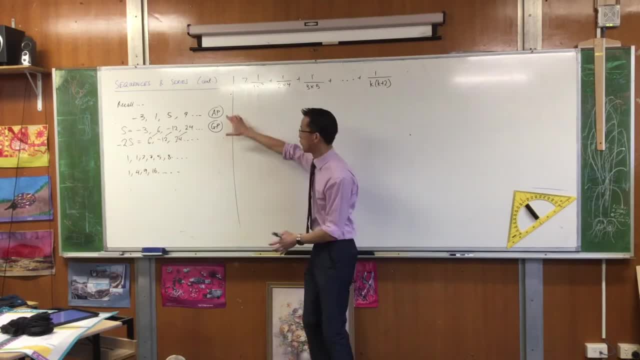 is to try and sense. all right, well, we used some tools before to sense the pattern here. right, we can do something similar to sense the pattern here if we can get something that will show us. oh yeah, you can pair these things up or you can cancel these things out. it won't be exactly. 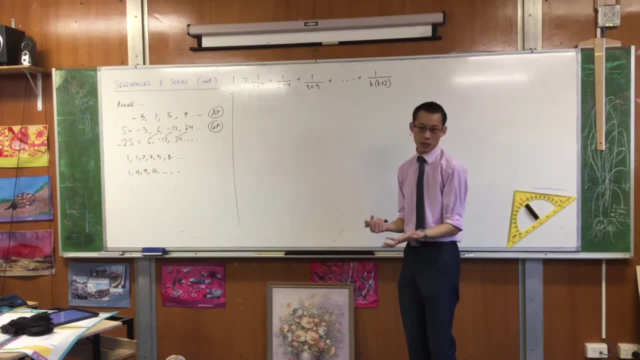 the same as these guys can still nap. it's not a gp, but there are other things we can do. so i want to take the problem, or the strategies, rather that i suggested right in the first lesson to try and look at this thing, and there are no words in it, but it's just as problem-solving and unfamiliar. 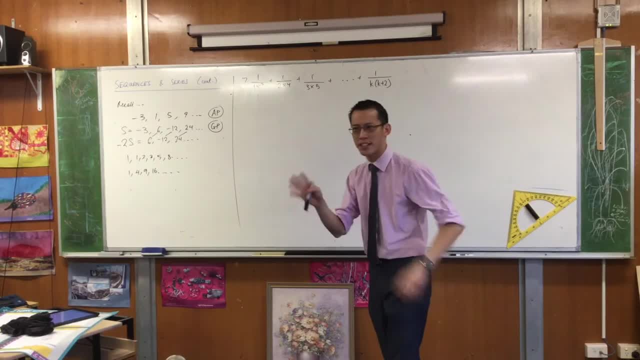 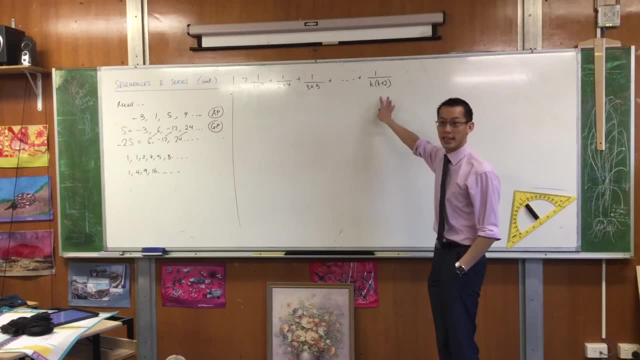 as that thing with um, what was it? the guy with three, three children and we had to try and work out their ages. do you remember that? in the violin right? so what kinds of things did we do there? well, i think the first thing was we wanted to dissect the problem. do you remember that? it just looks. 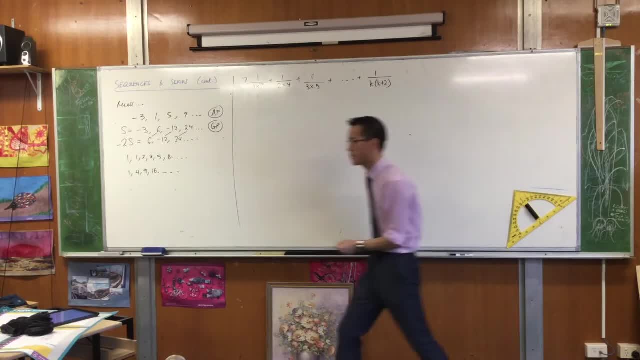 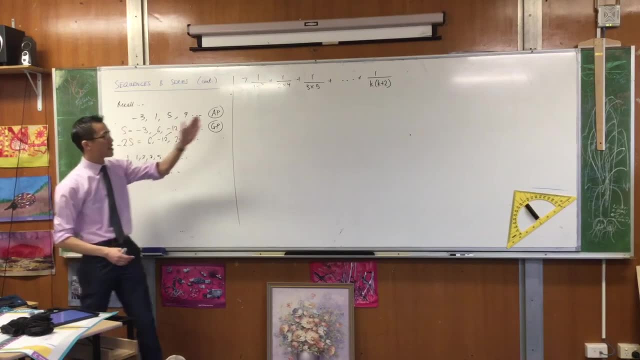 weird and imposing. so how can we break this down a little bit? okay, what i want to notice is a? um. a problem like this is always set up to be dissected because there's a an unknown number of terms, but every term looks the same. do you notice that they all follow a? 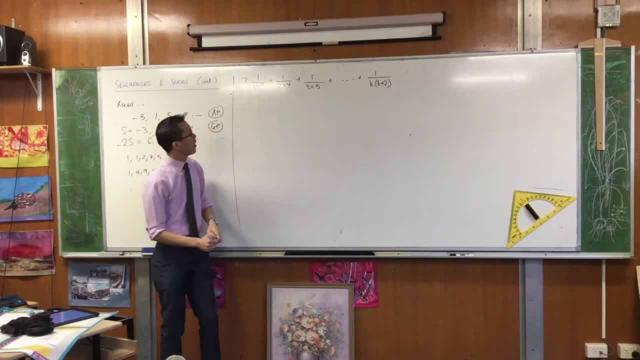 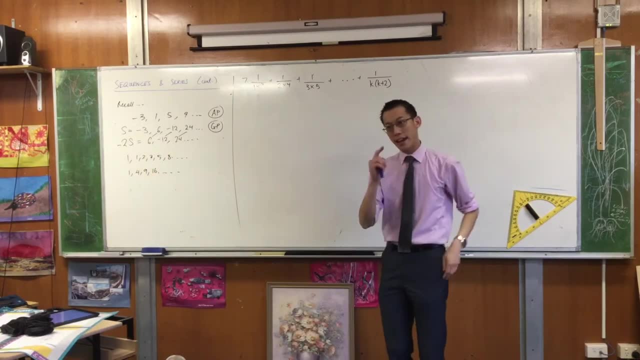 pattern, which is the whole idea of this one, and then this one, and then this one. how do you get from one term to the next? what do you do to advance from one term to the next? each one of those things are the denominators. by the way, we have language for this. rather than saying things what, what are? 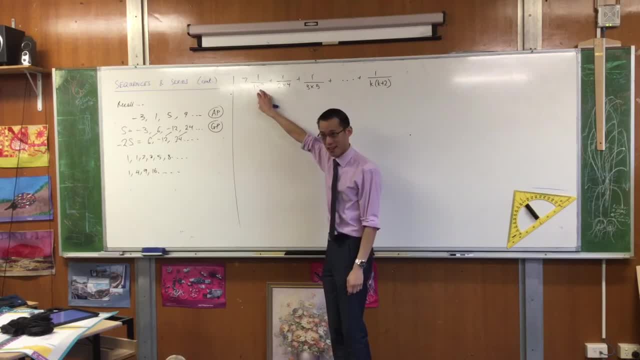 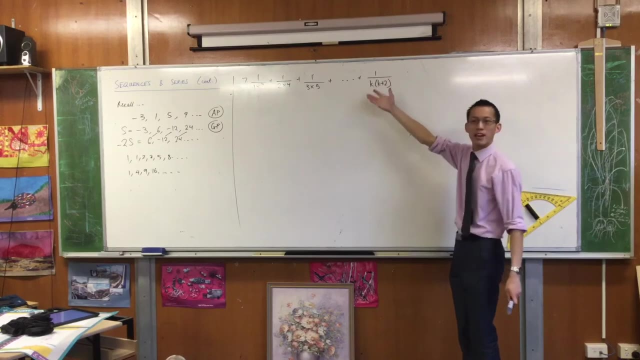 these things, they're factors in a product right. so each one of these factors, we add one to it, we increase it by one and it changes into this. and then each of these factors, we increase it by one, it turns into this. and you do it until such a time as you get to whichever value of k you like, the hundredth or 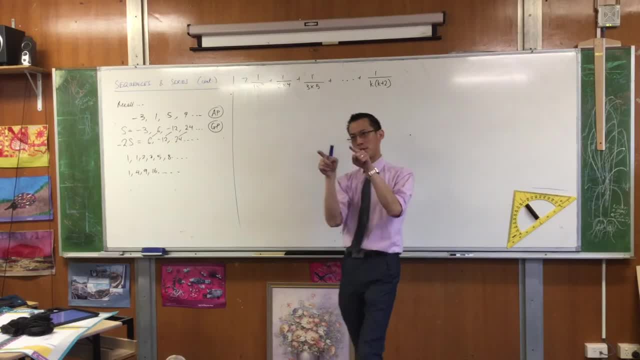 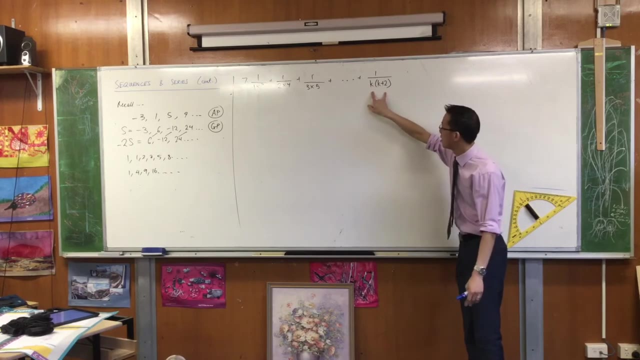 a thousandth or something like that, but because you're making each of the factors advance one right, the gap between the factors is always two, and the next one will be four and six, then the next one will be five and seven, and so on, which is why the kth term is k and k plus. 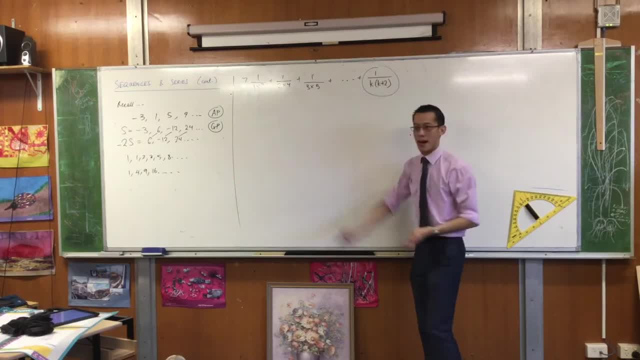 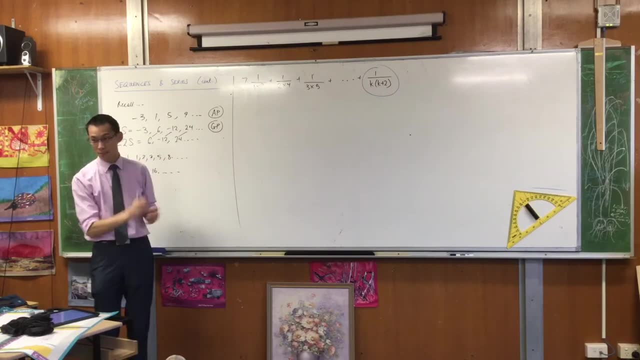 two. does that make sense? so what i want to do is just dissect it. let's just look at this guy. every single term is in this format, so how can i work out what's going on there? what makes this term, this term, okay? one over k, k plus two. i want you to consider something like this: 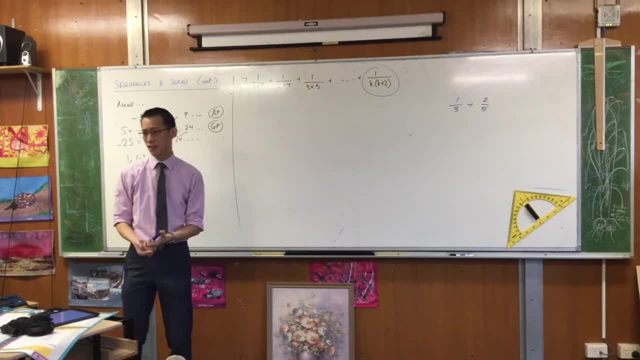 okay, if i added you, if i asked you to add these two factors together, what would be the first thing that you do? you would go for a common denominator, wouldn't you? so you're like, i can't get these two fractions to talk to each other in thirds and fifths. 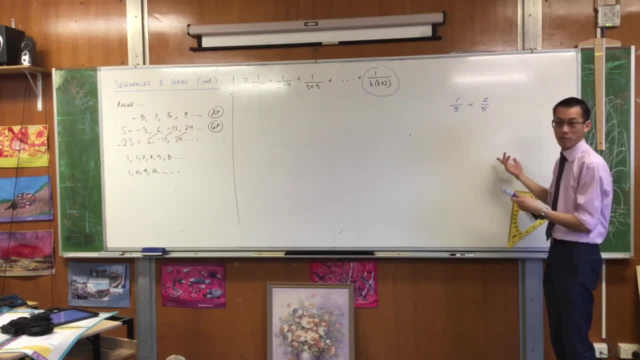 so i will get them to be in this case in 15th right. so in long form i would write this as 5 over 3 times 5.. i know that you know what that is. you can just go straight there, but i'm trying. 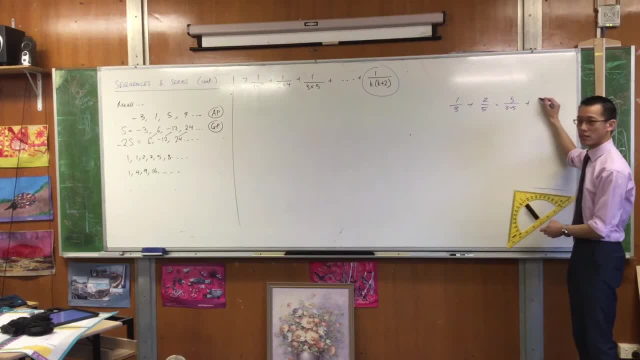 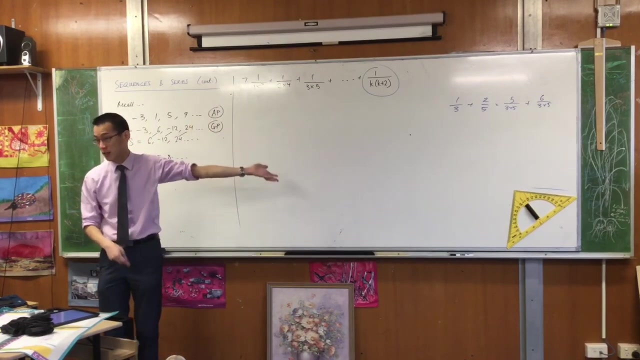 to point something out here, right, and then this guy you would write as what would you write? that, as it'd be six, over again, three times five, okay. so what i'm noticing is one of the primary reasons why you get fractions which have, like lots of things on the denominator, extra factors on the 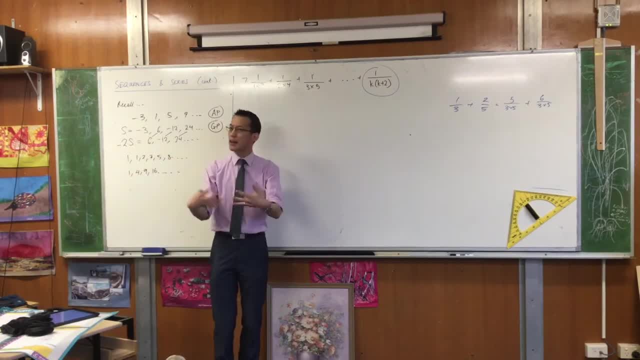 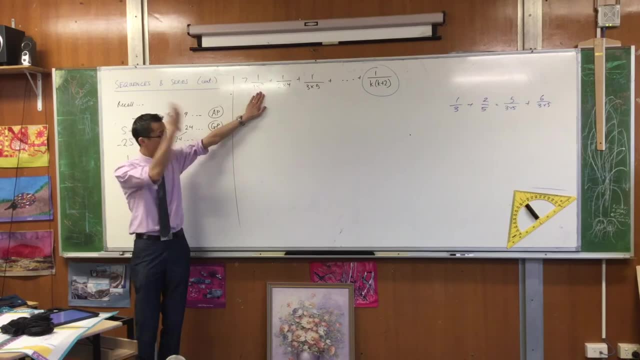 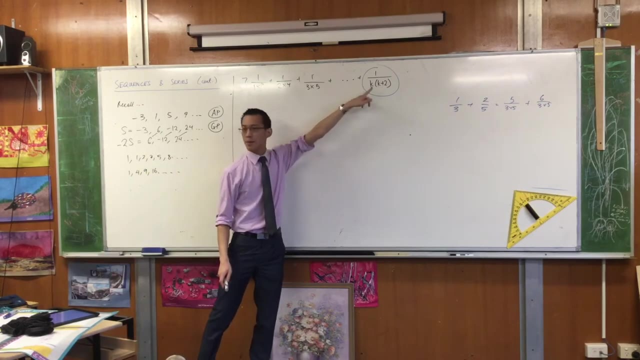 denominator like this is when you combine two fractions, right? if you were to add or subtract two fractions together, then you sort of have to do this by necessity. you multiply the denominators so you can get a common one, right? so if we think about this, one over k, k plus two. 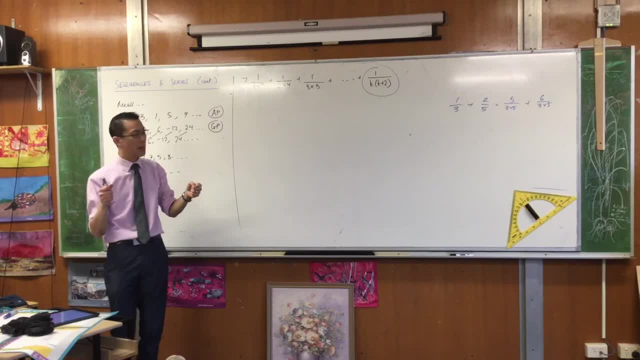 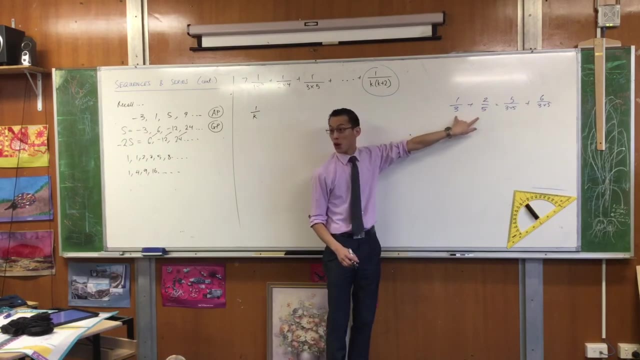 what kind of pair of fractions might this have come from? now, i don't know, so i'm just going to take a stab in the dark. this again is a classic problem solving strategy. just try something and see what happens. right at the very least. you see this guy here. it came from fractions with those denominators. 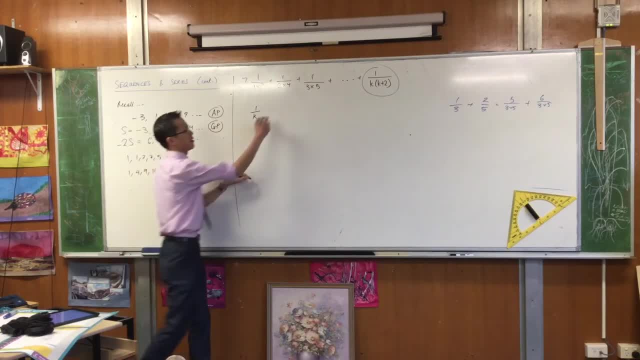 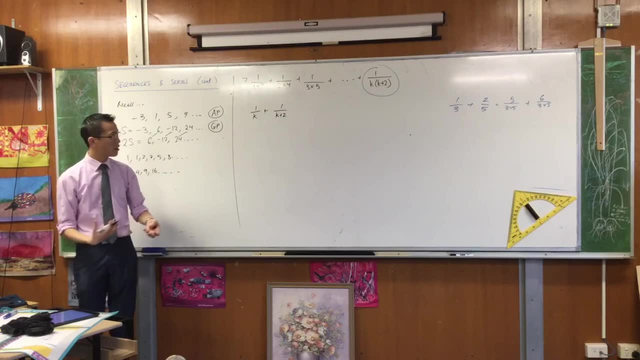 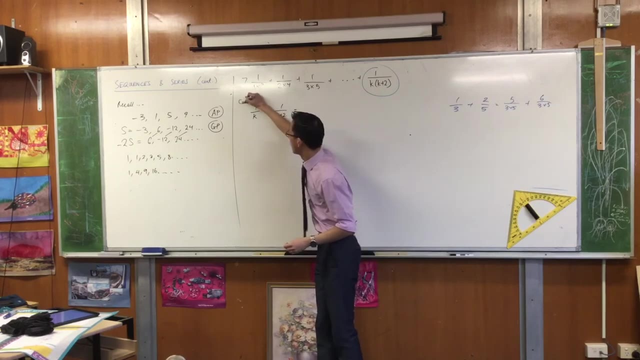 right. so why don't i try taking those guys, k and k plus two? here's a pair of fractions. it has those individual denominators, so when i put them together maybe i'll get something that looks like that. okay, so let's try it. when you add these two together, i guess i would say consider. 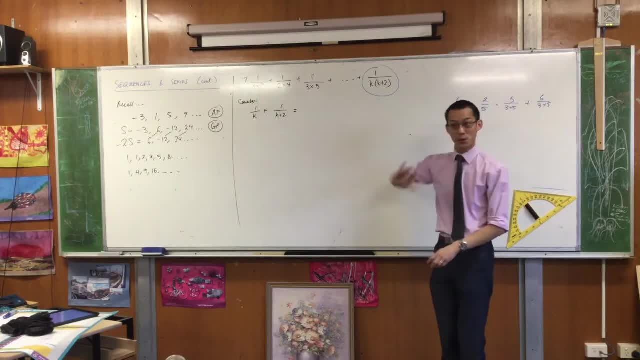 because i'm just trying to think this thing through and um, throw some things at the wall and see what sticks. okay, but they're not just random, it's an educated guess. what are you going to get? the common denominator is going to be k times k plus two, but what will this numerator 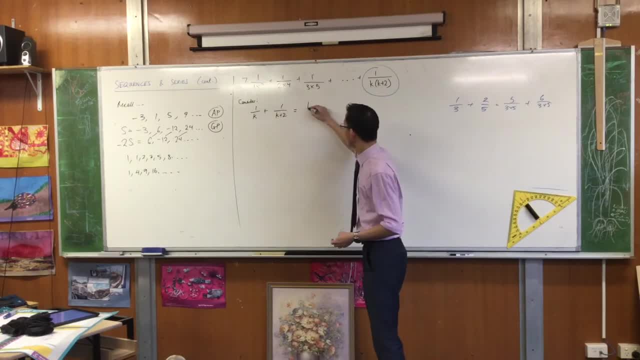 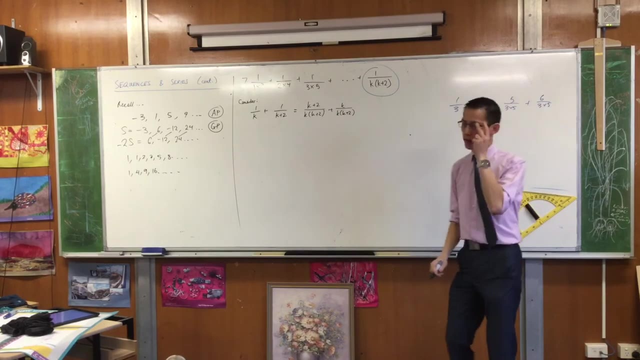 become the first, one k plus two. right, because that's what you want to apply the top and bottom by. what about the second fraction? okay, okay, now, when i have a look at this, this gets the denominator that i wanted, but i don't even need to go much further, like in terms of simplifying this numerator. you can see i'm going to get 2k plus 2. 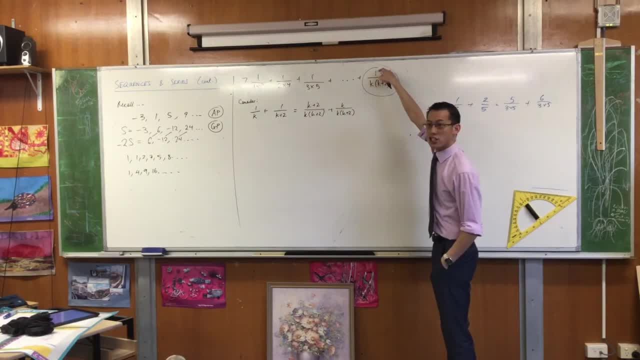 which looks nothing really like this. okay, 2k plus 2.. all i'm supposed to have is a number up there, no k's or anything like that. the k's have crept up because of multiplied vertices. so how would i overcome that? well, i add those fractions before i added them, which is why this is what i'm going to. 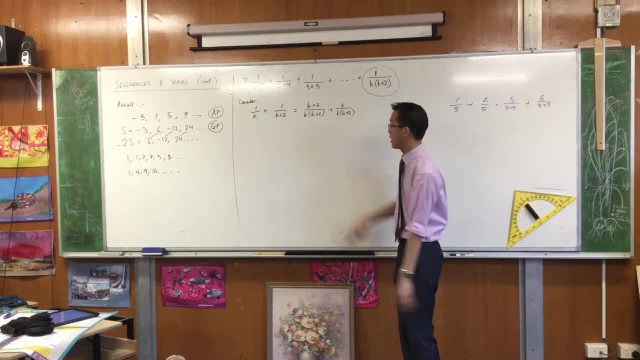 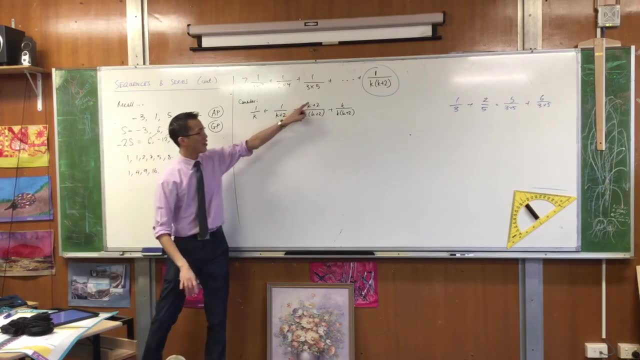 do now. so i'm going to do this and this combine in this unfortunate way, but that's not the only thing i can do. right, if i, if i don't want any k's on the top, do you see? there's a k here and a k there. 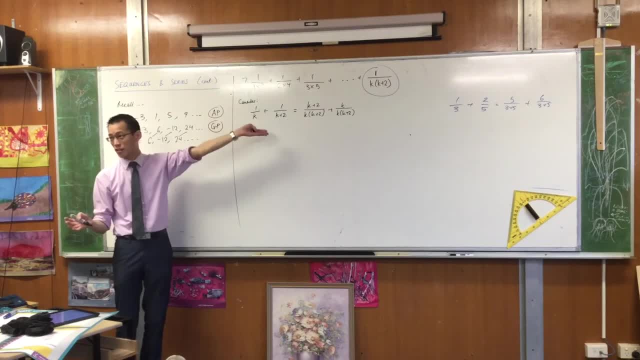 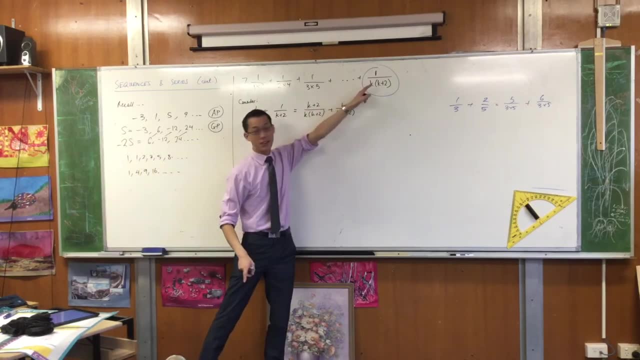 i can get them to actually cancel each other out, can't i? instead of adding the fractures together, why don't i try subtracting if i multiply? if i multiply, i do have this, but then i don't. i mean, when things are multiplied together i don't have something. that's much simpler than what i've. 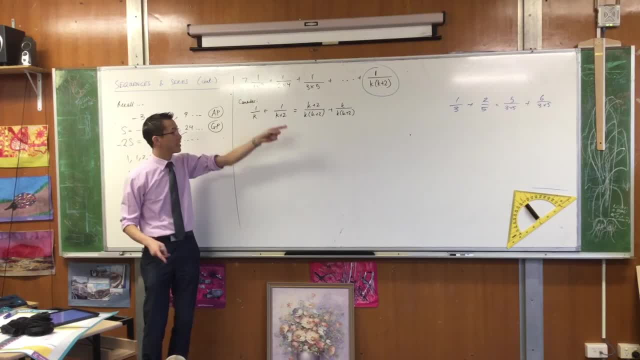 already got. okay, if i have something that's added up or subtracted. you see, this is added up and subtracted, so i'm hoping for something to cancel out, so i'm going to write the subtraction instead. let's try this. what is going to happen? well, it's going to be exactly the same thing, except with 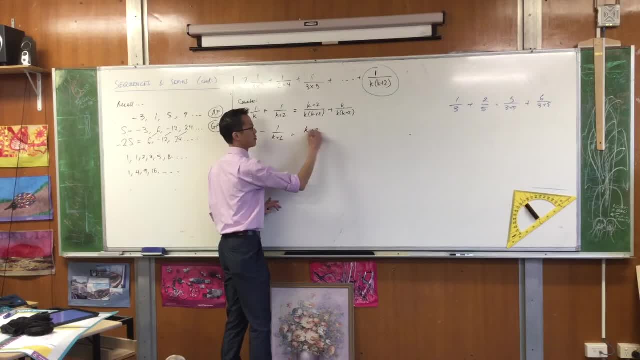 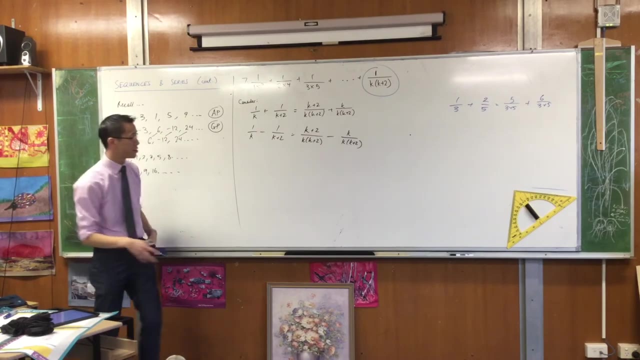 a minus sign instead of a plus sign, so i'm going to get this. okay. now this doesn't seem like it's all that helpful just yet, but let's poke on it and play with it a little bit. on the numerator, the k's are going to cancel. so what will you be left with? two. 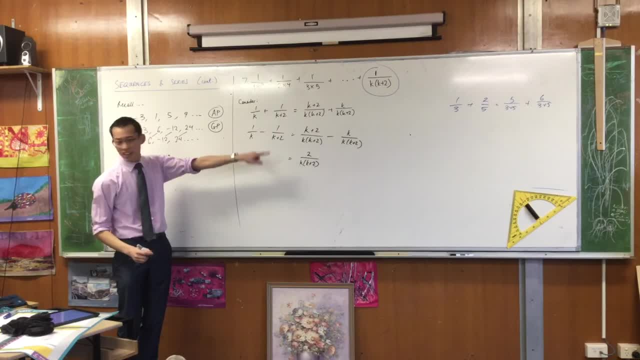 okay, it's two. i actually want one, don't i? that's what i really want. so, being that, this is what i started with. if it turns into a two on the numerator and i want it to be a one, i'm just gonna. it's an equation. 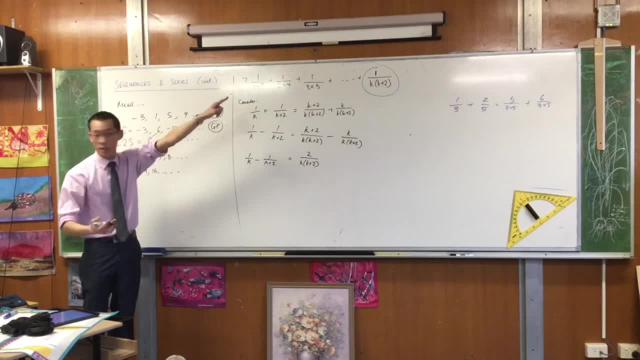 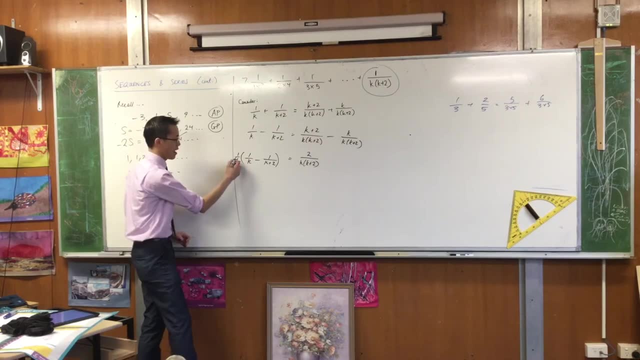 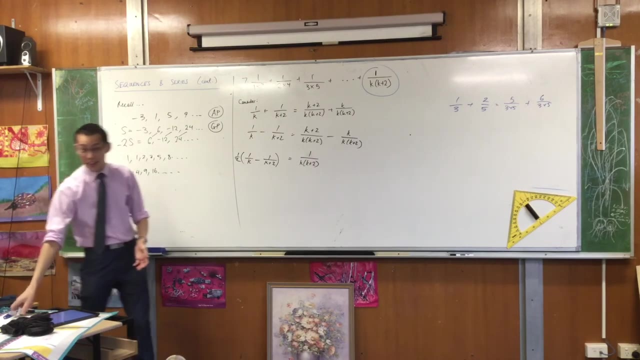 i'm just going to two. Does that make sense? And I'll get the theme that I want? So I'm going to divide this by two. I guess I'll just stick half at the front and that will turn this into one. Are you happy with that? Now I want you to again come back to a couple weeks. 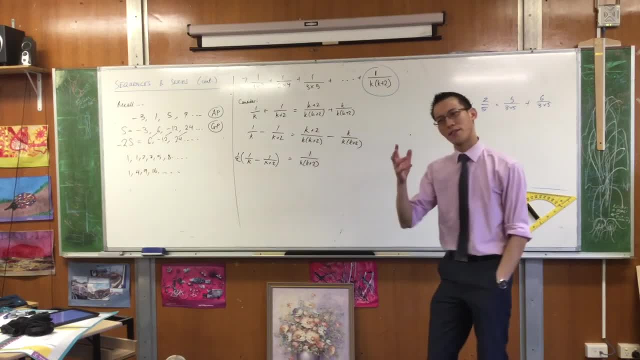 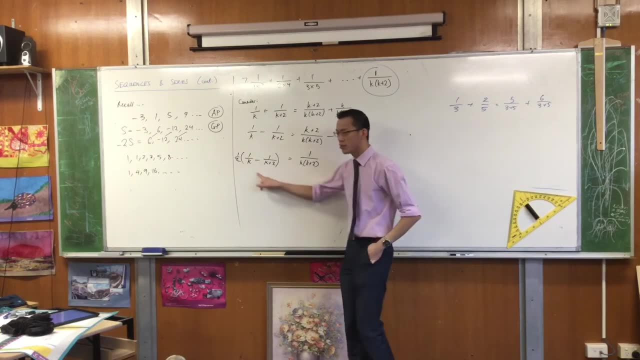 ago, Do you remember? we spent a long time on factorizing, Do you remember that? And we said factorizing was useful because you can reveal the structure of an object if you know its factors right. Well, I'm trying to do something a little bit in reverse. I'm